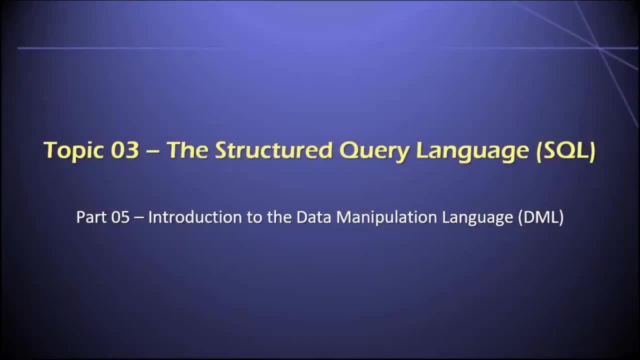 Hey everyone, welcome back In this video, part five of topic three in our database class, I'm going to provide a brief introduction to the data manipulation language, or DML, component of the broader structured query language. All right, so we will return a little. 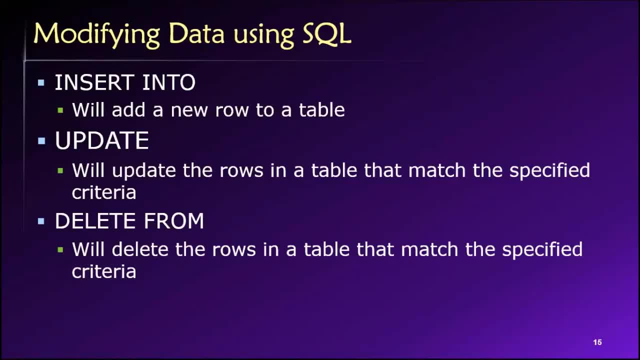 later in this topic back to the DDL, but for now this is a good time for us to transition into learning about three of the four operations that together comprise the DML, part of the structured query language. And, as a reminder, the DML means data manipulation. 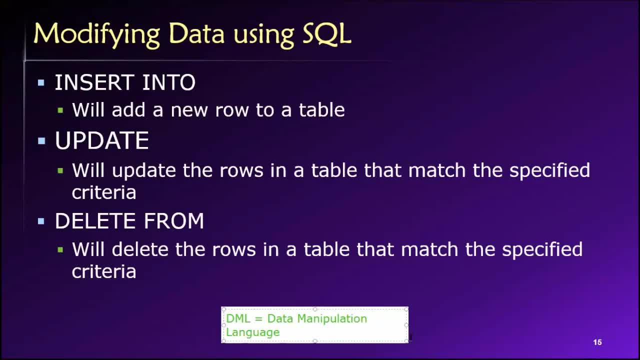 language. These are the commands in SQL server, or I should say in SQL, that allow us to do the data manipulation language, And these are the commands that allow us to allow us to do the data manipulation language, And these are the commands that allow us to. 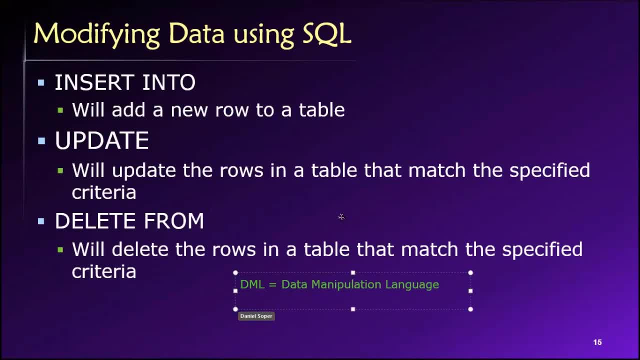 allow us to do the data manipulation language, And these are the commands that allow us to actually change or work with the data in the database. So as, in contrast to the DDL, the data definition language, where we were focused on structure, now we're focused on data. So it's 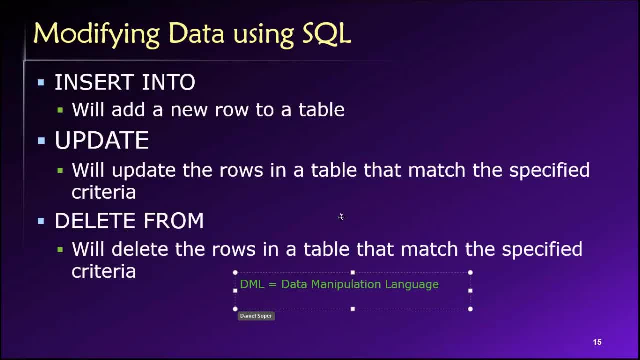 not the structure of the tables, but the data contained inside those tables. That's what the data manipulation language is all about, And there are four basic data operations that are handled by the data manipulation language, And they are creating new data. Let me change this color here. 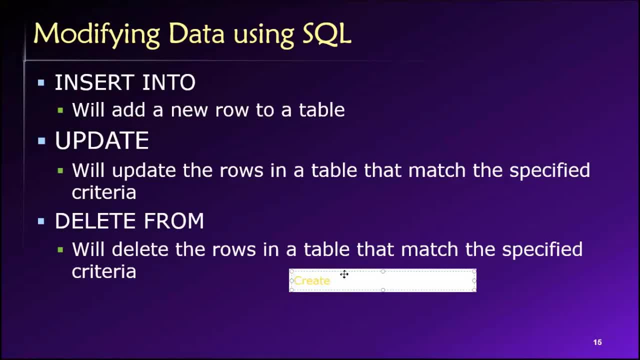 So creating new data, reading existing data, like getting values out of the database, updating existing data or deleting existing data. So these are our four basic data operations, And the reason I listed them like this is because it creates this acronym CRUD, which hopefully is something.